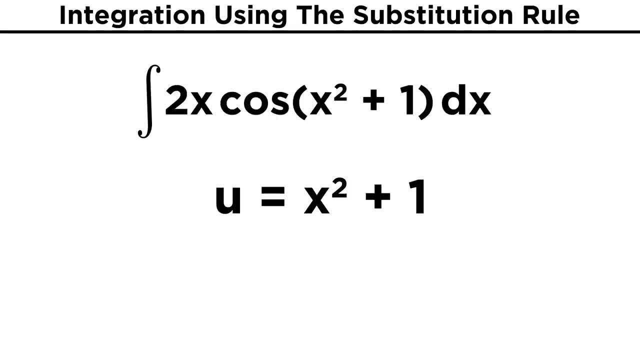 so nothing we have learned so far will work here. But let's try something clever. What if we make a substitution? Let's replace X squared plus one with the letter U. We are still saying the same thing, since U equals X squared plus one, but we are simplifying. 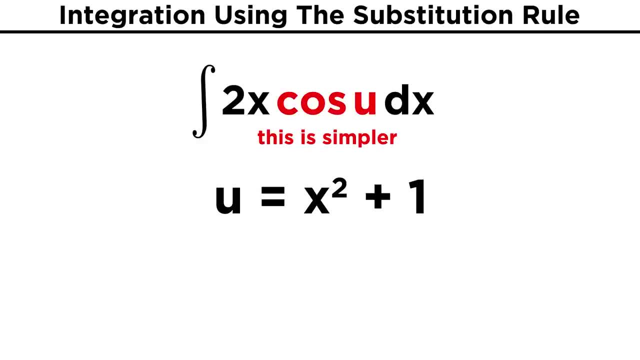 the integrand this way, because if cosine is operating on a lone variable rather than an expression, we will be able to integrate it. The only problem is that if we are changing things to U, this DX will be a problem. We need things in terms of U now, so we need this to be DU instead. 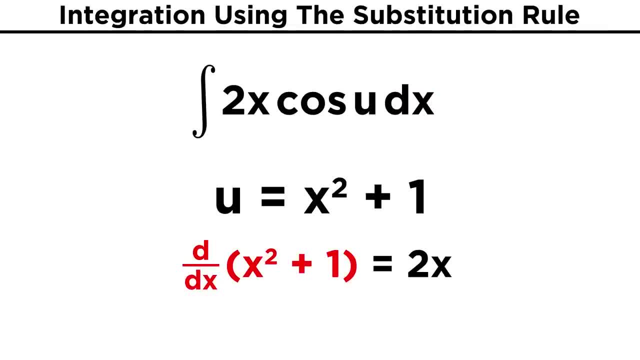 But we can fix that. Let's understand that D over DX of X squared plus one, or the derivative of this function with respect to X is two X. Now we can do something tricky. Let's bring the DX up to the other side to get two X DX. 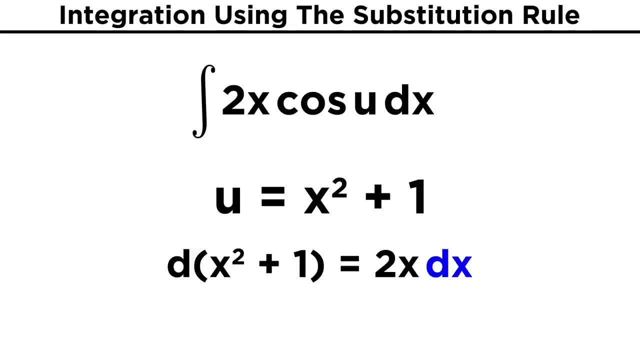 This may seem strange, as DX is simply part of the notation D over DX, and it may not look like something we can manipulate algebraically. Later in this series we will justify why this is possible. For now, let's just do it and observe how this is useful. 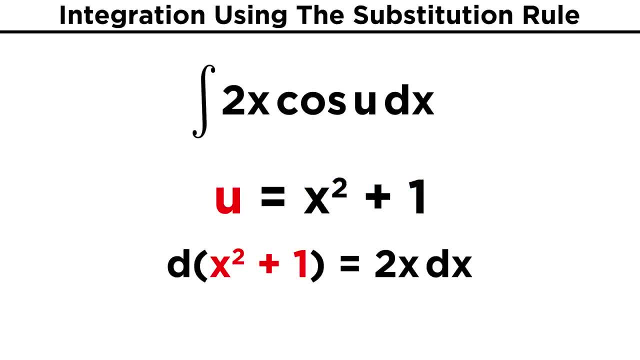 Now we can understand that the derivative of this function is the derivative of the derivative of this function. Now we can understand that this function on the left is what we are representing as U, so let's just change that to U and we therefore see that DU equals two X DX. 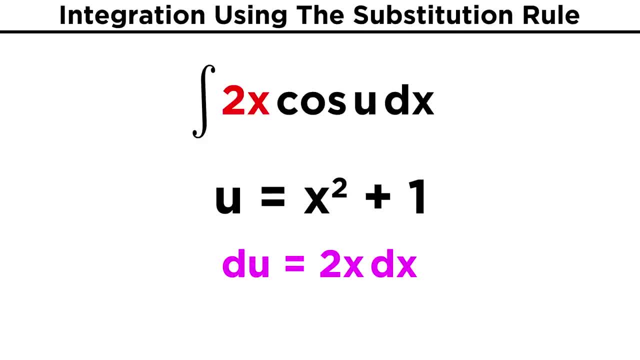 That's quite convenient because, lo and behold, if we bring the two X inside the integrand to the other side of this cosine term, we have two X DX right here. so according to this equation, we can just rewrite that as DU. 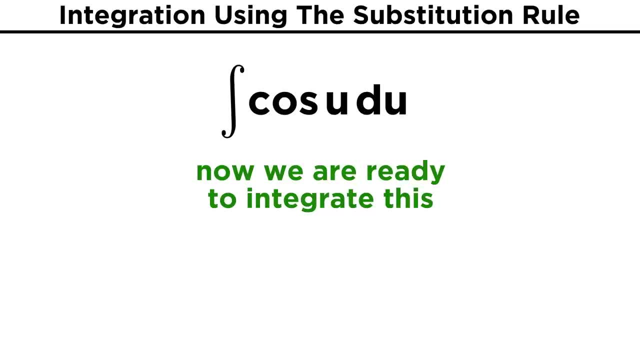 Now that we have a differential, we can just rewrite that as DU. Now that we have a differential DU that agrees with the rest of the integrand, we are ready to integrate. and cosine U DU can be integrated just like cosine X DX or cosine Z DZ or 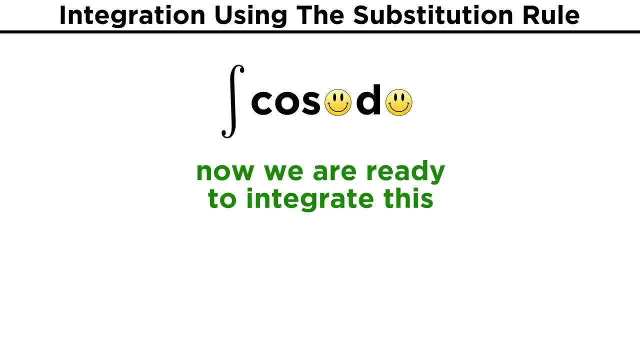 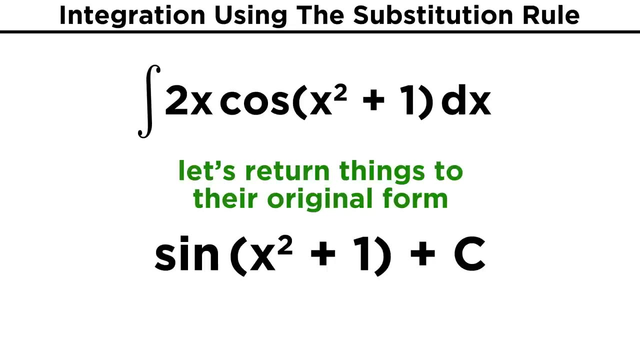 cosine smiley face, D smiley face. The variable doesn't matter. The integral of cosine U DU is sine U plus C. Now that integration is complete, let's return U back to its original form And we have sine of X squared plus one plus C, And that's the answer. 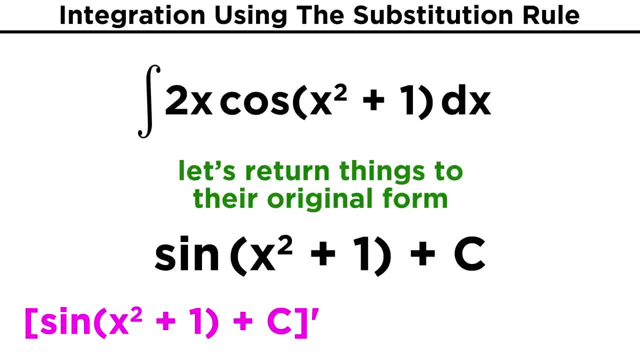 Just to be thorough, let's differentiate this and make sure we get what we started with. C will go away, so it's just sine of X squared plus one. According to the chain rule, we do the outer function first, so we get cosine X squared. 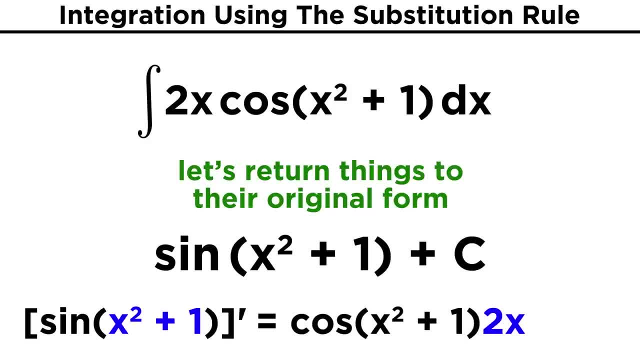 plus one times the derivative of what's inside, which is two X. That is indeed what we started with, So this approach worked like a charm. In this way, we can think of the substitution rule as the chain rule in reverse, because 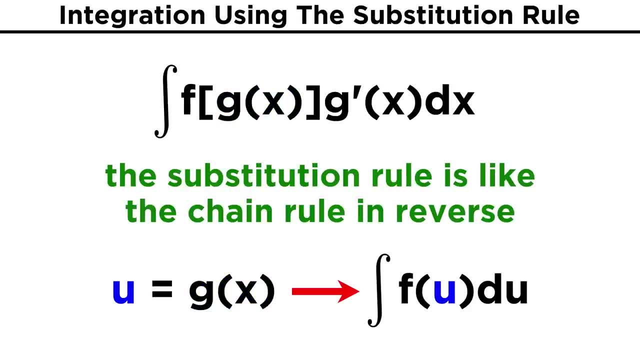 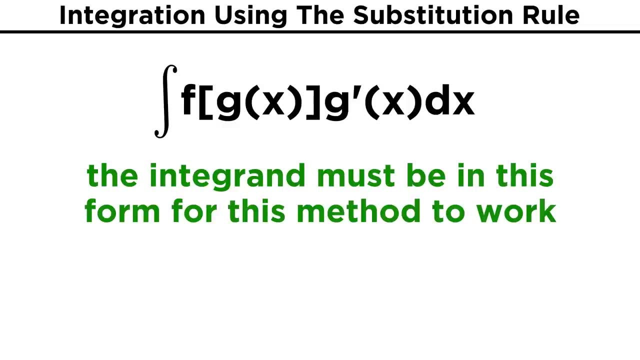 we symbolize some piece of the function with a single variable, allowing us to integrate more simply just the way that the chain rule ignores the inner function. during the first step of differentiation, The only thing to remember is that, while the chain rule will always work, the substitution 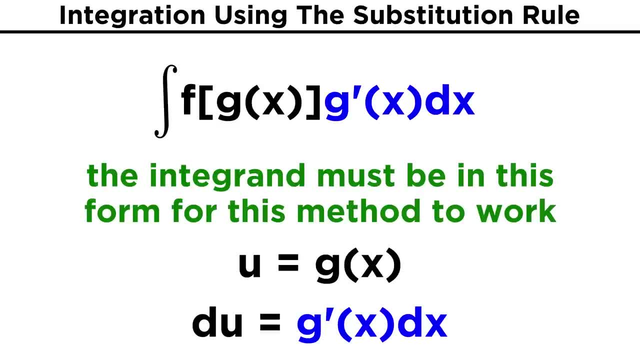 rule won't always work. It only worked here because our expression for DU was indeed present in the integrand, because the integrand was in the form F of G, of X times G, prime of X. If this wasn't the case, we couldn't do this, so we have to be able to look at an 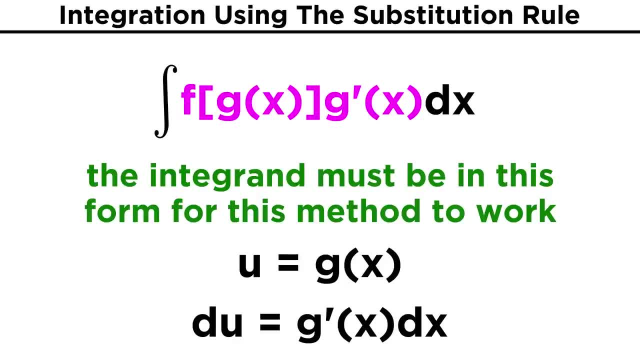 integral and recognize whether or not the substitution rule can be applied. If we do have an integrand in the form of F, of G, of X, then we can't do this. We have to be able to look at an integral and recognize whether or not the substitution 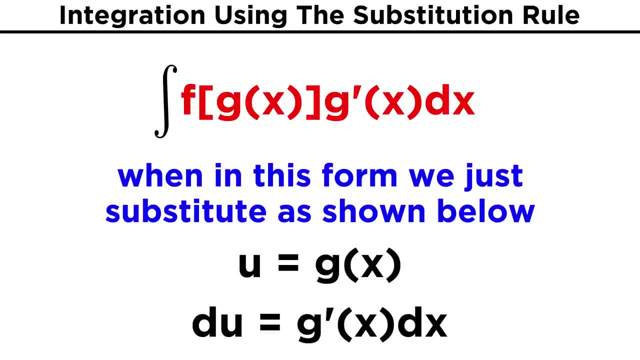 rule can be applied. If we do have an integrand in the form G of X times G prime of X DX, we can represent G of X as U G prime of X DX turns into DU and we end up with F of U DU, which we can. 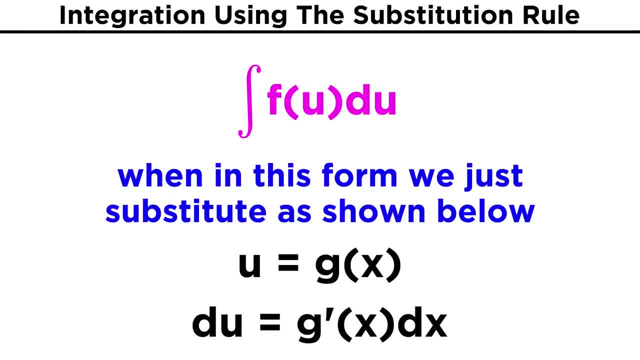 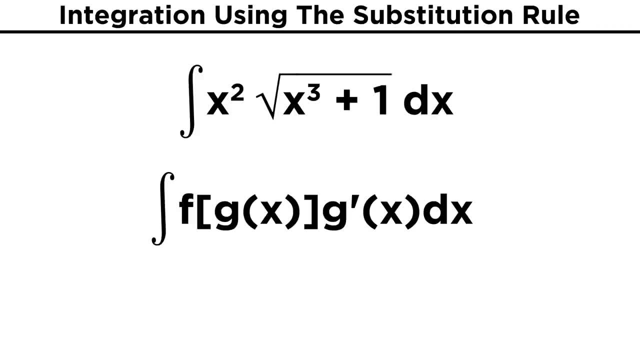 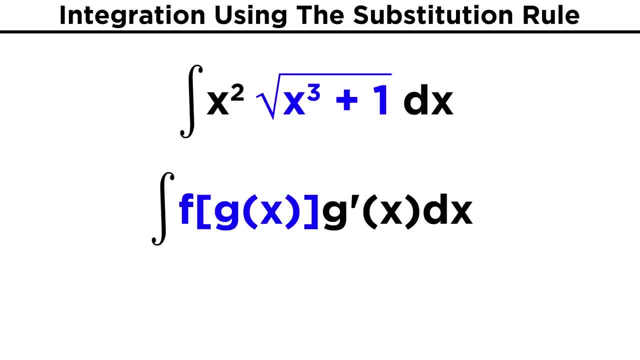 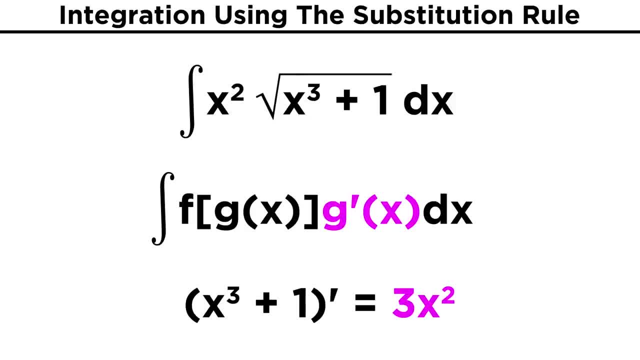 Well, G prime would be three X squared, and we pretty much have that. so let's give this a try and see what happens. Let's change X cubed plus one into U, so that we have root U, Now DU over DX, which means that we are differentiating the expression that U represents, with respect. 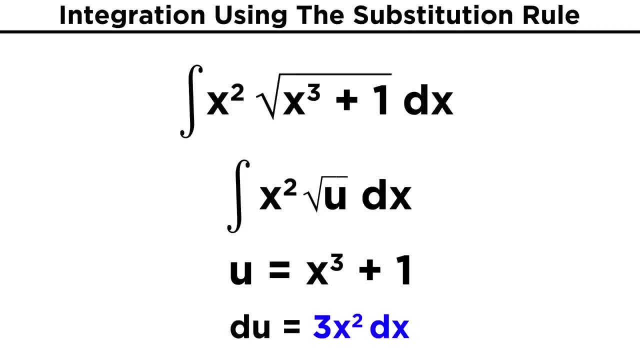 to x will equal three x squared. That means that du equals three x squared dx. Now, it's true that we don't have three x squared dx, but that's no problem, We have x squared dx, so let's just bring the three over to the other side. 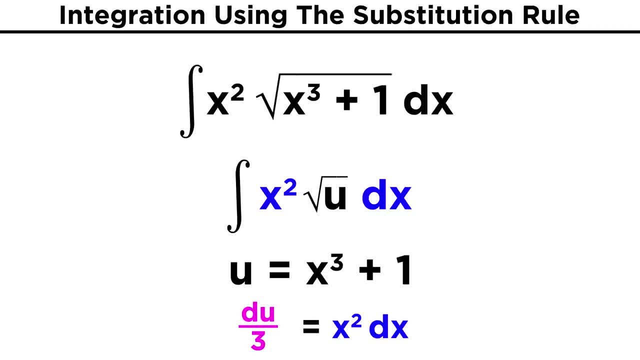 X squared dx will then equal du over three or one third du, So let's write one third du in its place. Now things are looking pretty good. let's pull one third out of the integral and then we can integrate root u du. 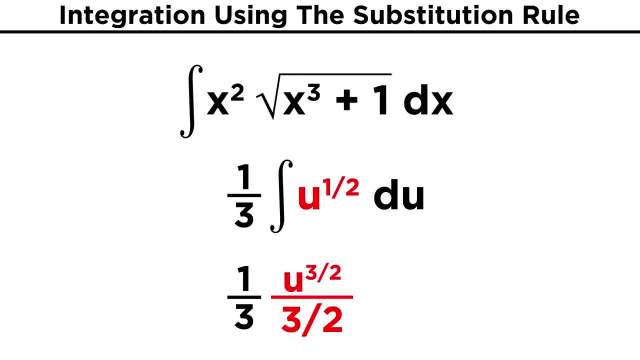 Remember that's u to the one half, so it will become u to the three halves, over three halves, or two thirds: u to the three halves times the one third we already had, and that will be two ninths: u to the three halves. 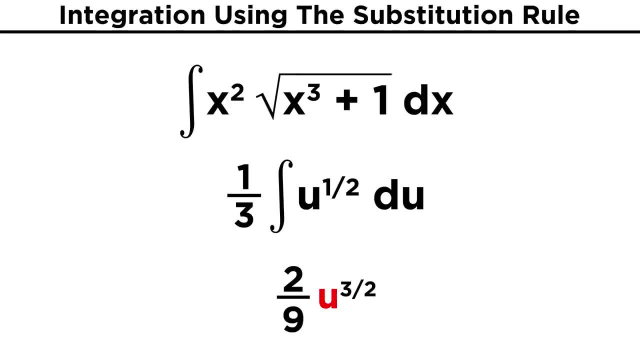 Now we can return u to its original form and we have two ninths times the quantity x, cubed, plus one to the three halves power, and then plus c, as we are used to. Let's do a couple with trig functions. How about sine to the sixth x times, cosine x, dx. 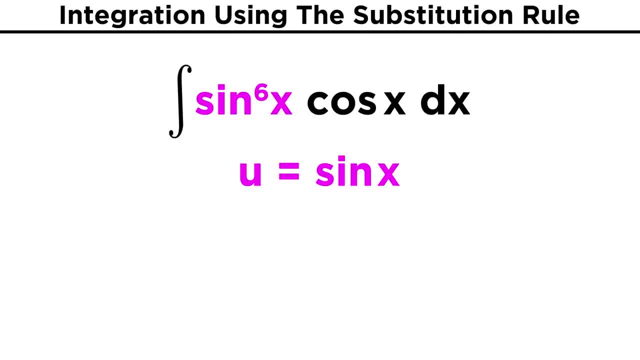 The sine term has more going on with it. so why don't we try representing sine x as u? Remember sine to the sixth x times cosine x dx. Remember sine to the sixth x times cosine x dx. The sine to the sixth x just means the quantity of sine of x raised to the sixth power. 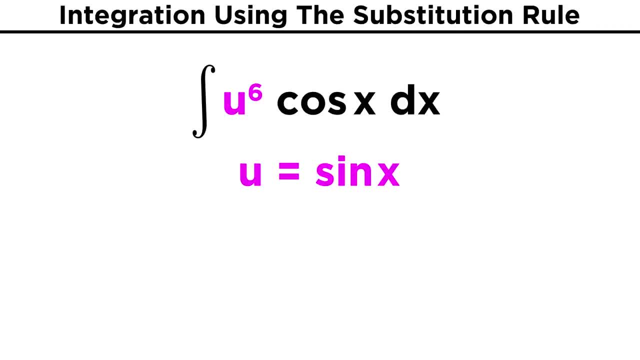 So this just becomes u to the sixth. Then du over dx equals cosine x. so du equals cosine x, dx. That is indeed present. so let's just make the rest of this equal to du, and we are ready to go. Integrating u to the sixth gives us u to the seventh over seven. 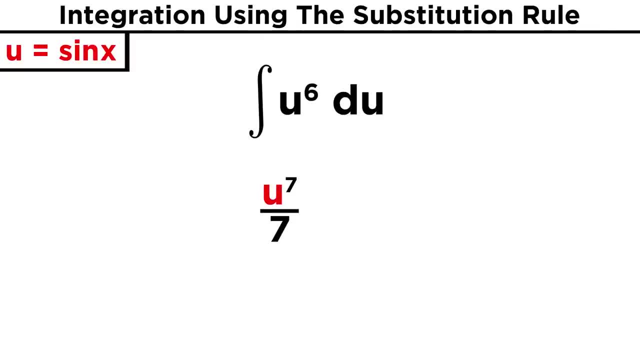 So that's u to the sixth. We return u to its original form and we get sine to the seventh of x over seven plus c. Now how about tangent x, dx? This is an example where substitution might not jump out immediately as a possible strategy. 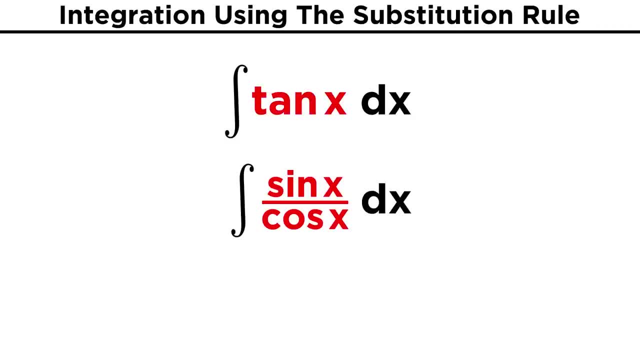 but if we remember that tangent is sine over cosine and that the derivative of cosine is negative sine, then we might see a plan unfold. Let's use cosine x as our u, and that means du will be negative sine x, dx. We have positive sign, so let's make this negative du and then pull the negative sign. 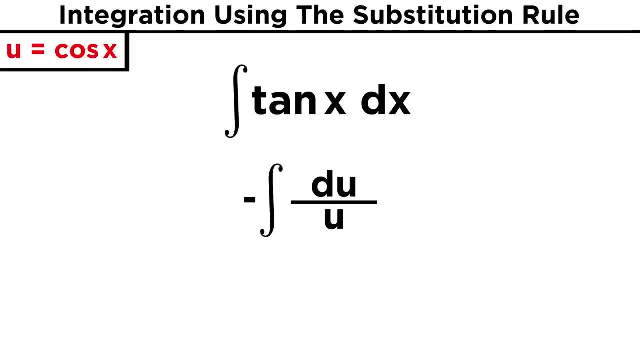 out Now: du over u is the same as one over u times du, and we know that the integral of one over u will be the natural log of u. I'm going to figure this out myself. Listen U in absolute value brackets, because this value will sometimes be negative as it's. 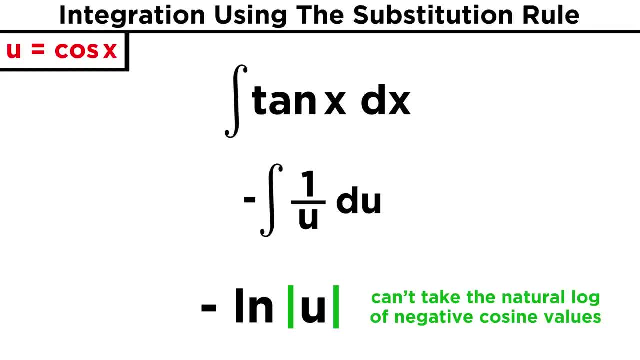 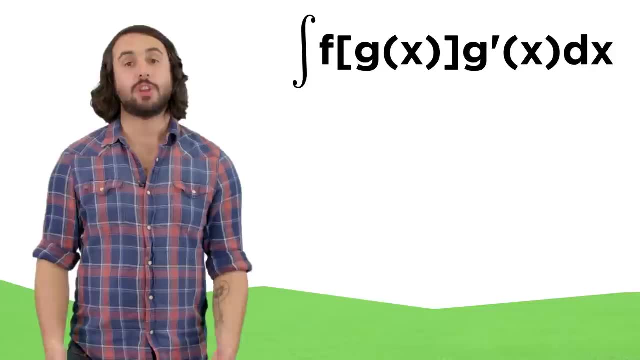 a cosine function and we know that the natural log can't take negative values. So we get negative natural log of the absolute value of U plus C and then change U back to cosine and that's our answer. So remember, any time we are integrating some function and the function can be split up. 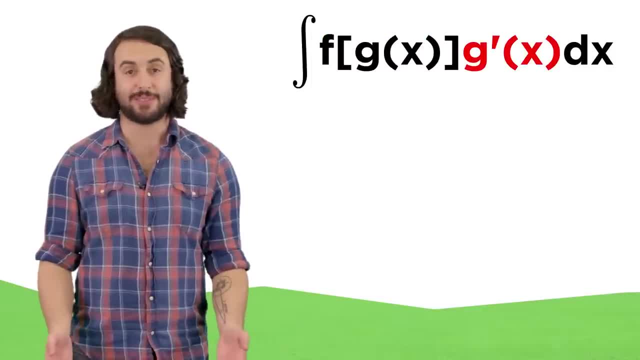 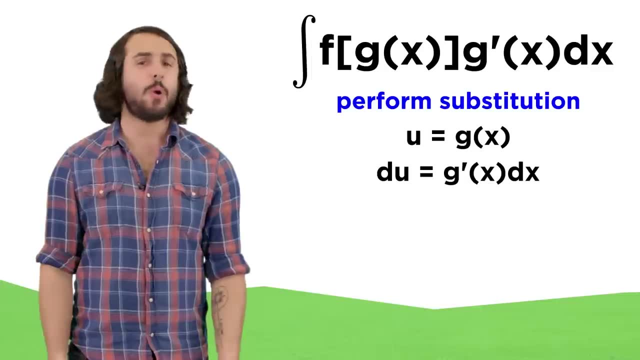 into a smaller function, followed by the derivative of that smaller function or something very close to it. the substitution rule is a good idea for something to try. This won't always work, but if it does it can take a complicated integral and make. 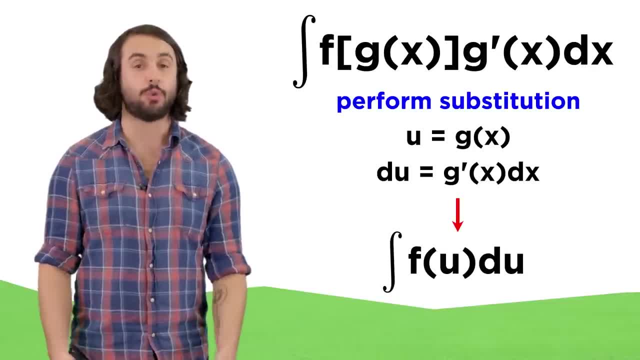 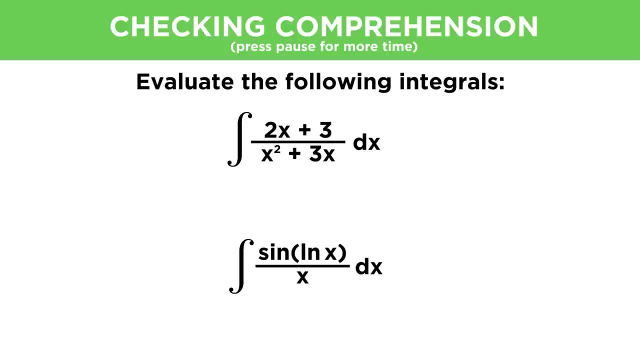 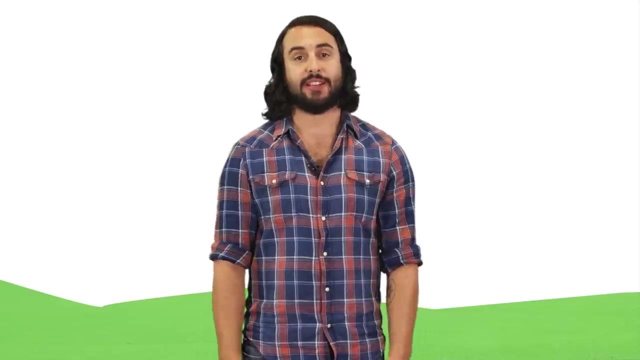 it very simple, so it is definitely a great start to our bag of tricks for integration. Let's check comprehension. Thanks for watching, guys. Subscribe to my channel for more tutorials, Support me on Patreon so I can keep making content And, as always, thanks for watching. Feel free to email me, professordaveexplains at gmail dot com.